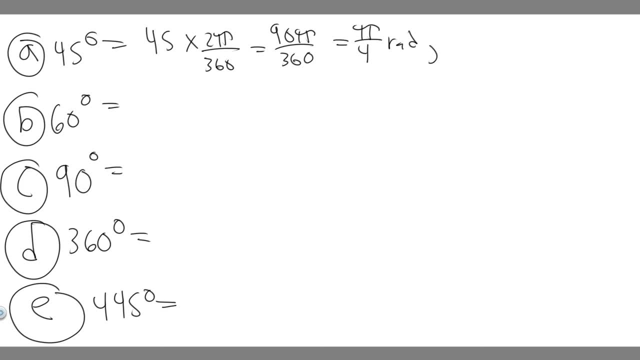 it as a decimal, So you just want to plug it in your calculator. So just do pi divided by 4, and you'll get 0.78539, and so on. I'm just going to round to 0.785. 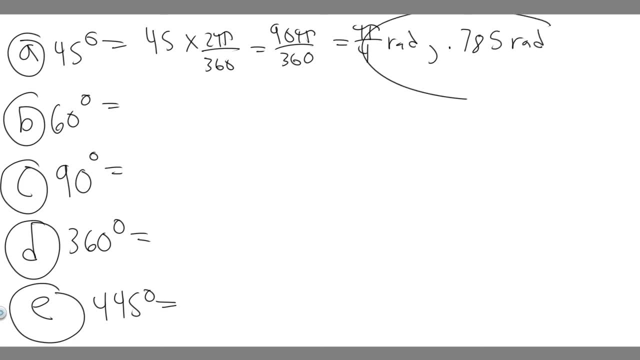 So 0.785 radians. But yeah, so this right here is a, so let's move on to b. So I'm going to go a bit faster. So 60, and then multiply by 2 pi over 360.. 2 times 60 is 120.. So 120. 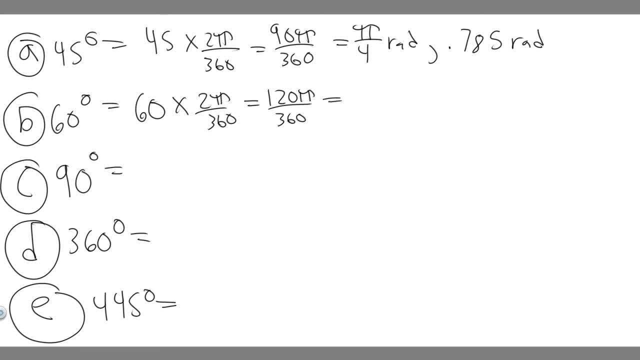 pi over 360.. If we divide both by 120, this is going to be 1, this is going to be 3.. So it's just pi over 3.. And if you're familiar with the unit circle you should know this. but you probably learned. 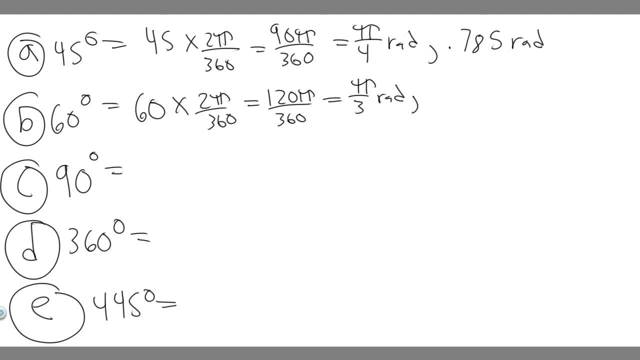 this back in pre-cal. but yeah, So pi over 3 radians and then just go ahead and plug it in your calculator and divide by 3.. So pi over 3, it's going to be 1.047.. So I'm just. 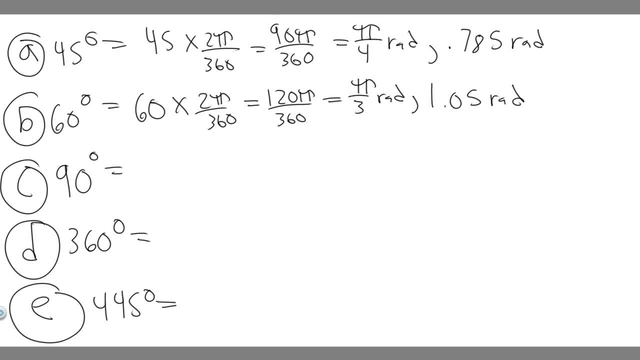 going to round to 1.05, and then radians. So 90 times multiply by 2. pi over 360. This is going to be 180 pi over 360. Which is just going to be pi over 2, right, Divide both by 180.. So pi over 2 radians. 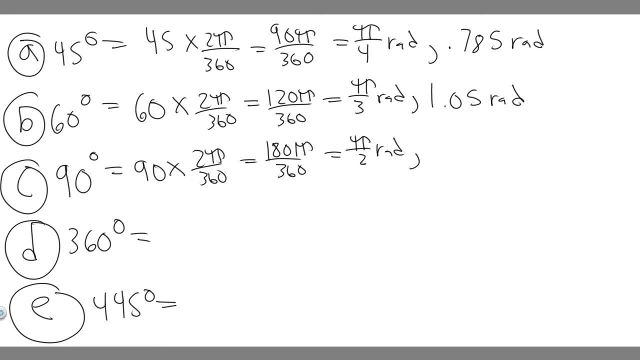 and then plug this in your calculator: 1.5707.. I'm just going to round to 1.57.. So 1.57 radians 360, 360 times 2 pi over 360.. Notice that these just cancel. So you're just going to. 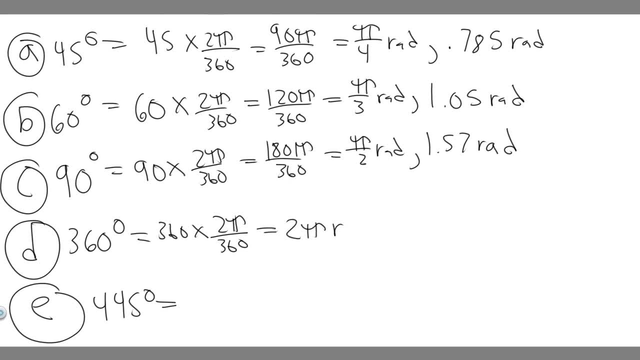 get 2 pi right. So it's going to be 2 pi radians, And then you're just going to get 2 pi over 360. And then you're just going to get 2 pi over 360. And then you're just going to get 2 pi over 360.. 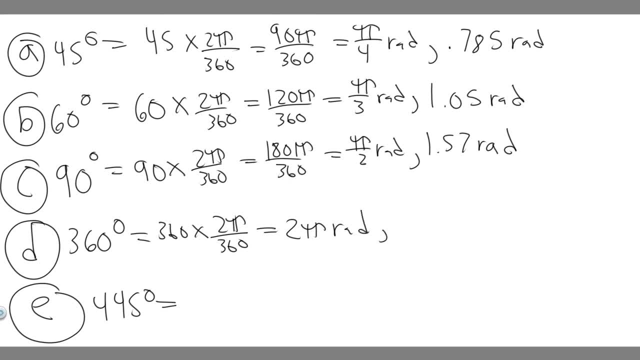 And then do 2 times pi, You're going to get 6.2831.. I'm just going to round to 6.283 radians. Now let's do 445.. So 445 times 2 pi over 360.. So if you go ahead and do this, right,